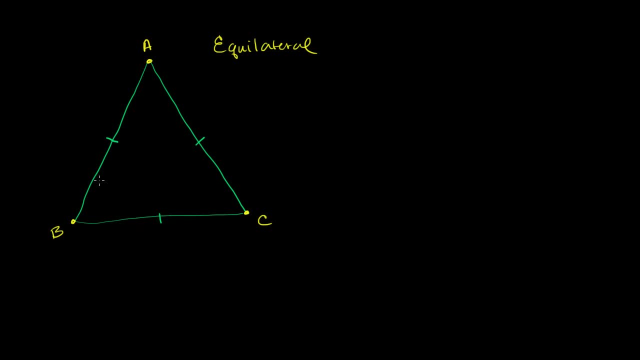 And we know for isosceles triangles, if two legs have the same length, then the base angles have the same length, And then so let's write this down- We know that triangle ABC is going to be congruent to angle ACB. 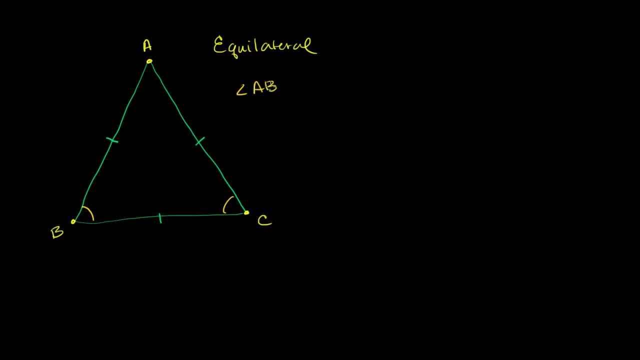 So let me write this down: We know angle A BC is congruent to angle ACB, because so maybe this is my statement right over here, Statement. And then we have reason, And the reason here, and I'll write it in just kind of shorthand. 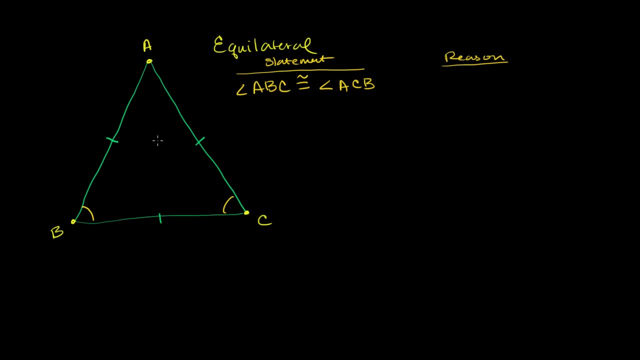 is that they're base angles of, I guess you could say, an isosceles, Because we know that this side is equal to that side. Now, obviously, this is an equilateral- All of the sides are equal, But the fact that these two legs are equal, 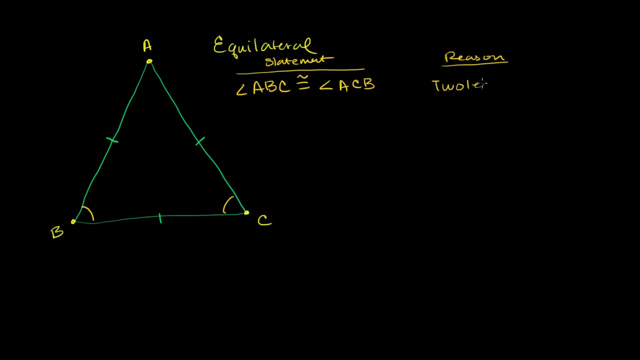 show that the base angles are equal. So we say two legs equal imply base angles are going to be equal. And that just comes from what we actually did in the last video with isosceles triangles. But we could also view this triangle the other way. 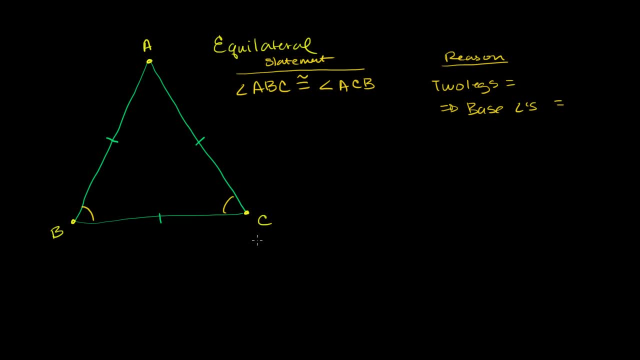 We could also say that maybe this angle over here is the vertex angle, Maybe these two are the base angles, Because then you have a situation where this side and this side are congruent to each other, And then that angle and that angle are going to be base angles. 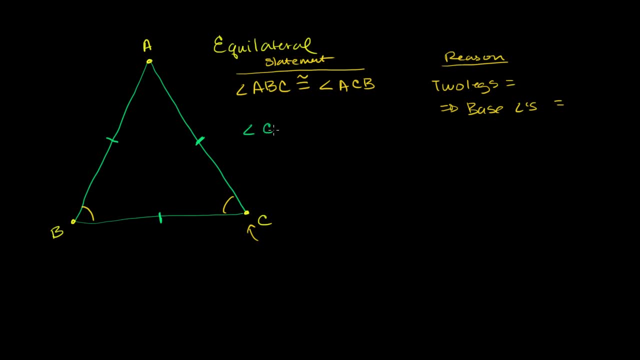 So you could say: angle CAB is going to be congruent. So angle CAB is going to be congruent to angle ABC. Really, for the same reason, We're now looking at different legs here and different base angles. This would now be the base in this example. 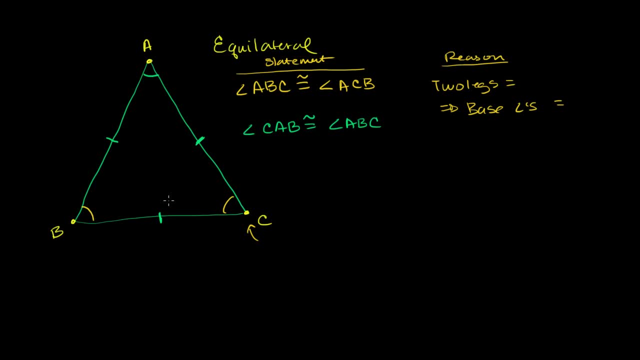 You could imagine turning an isosceles triangle on its side, But it's the exact same logic. So let's just review what I talked about. These two sides are equal, which imply these two base angles are equal. These two sides being equal imply these two base angles. 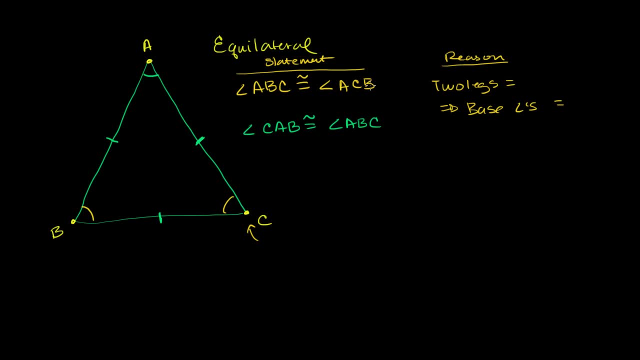 are equal. Well, if ABC is congruent to ACB and it's congruent to CAB, then all of these angles are congruent to each other. This is congruent to angle ACB, which is congruent to angle CAB, And that pretty much gives us all of the angles. 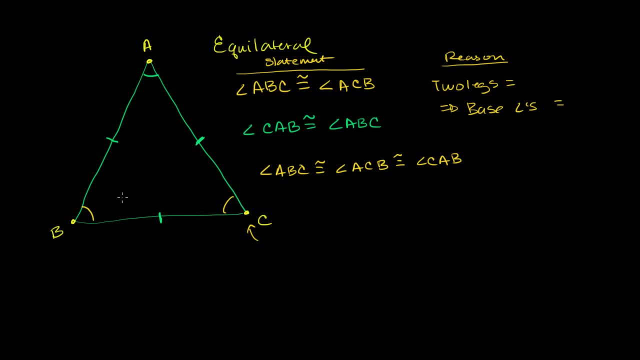 So if you have an equilateral triangle, it's actually an equiangular triangle as well. All of the angles are going to be the same, And you actually know what that measure is If you have three things that are the same. so let's call that x, x, x, and they add up to 180,. 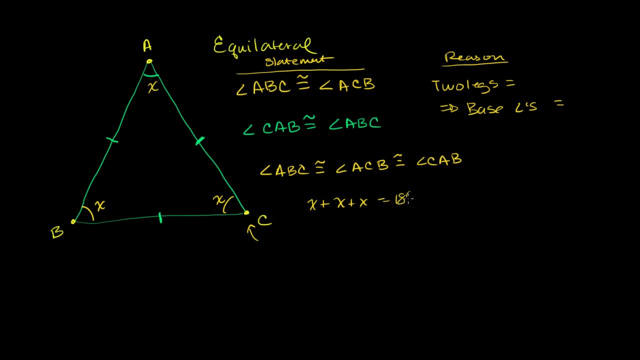 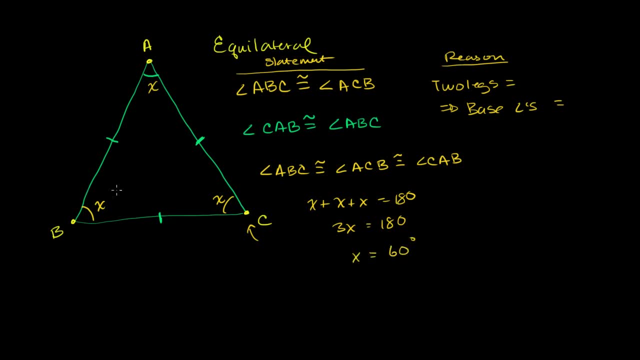 You get: x is equal to 60 degrees. So on an equilateral triangle, not only are they all the same angles, but they're all equal to exactly. They're all 60 degree angles. Now let's think about it the other way around. 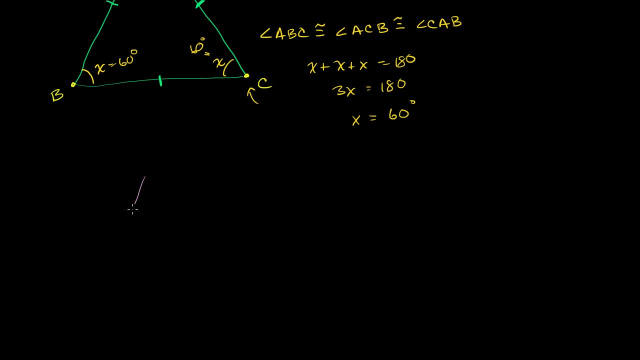 Let's say I have a triangle. Let's say we've got ourselves a triangle where all of the angles are the same. So let's say that's point x, point y and point z, And we know that all the angles are the same. 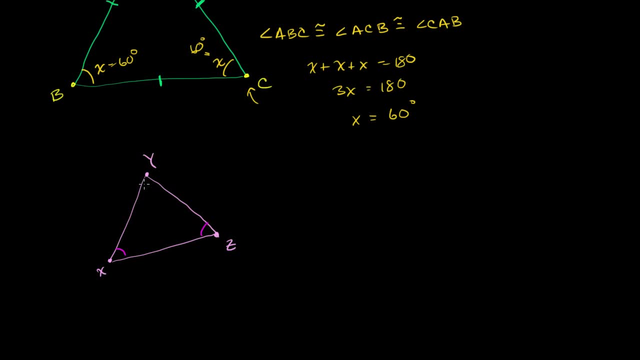 So we know that this angle is congruent to this angle is congruent to that angle. So what we showed in the last video on isosceles triangles is that if two base angles are the same, then the corresponding legs are also going to be the same. 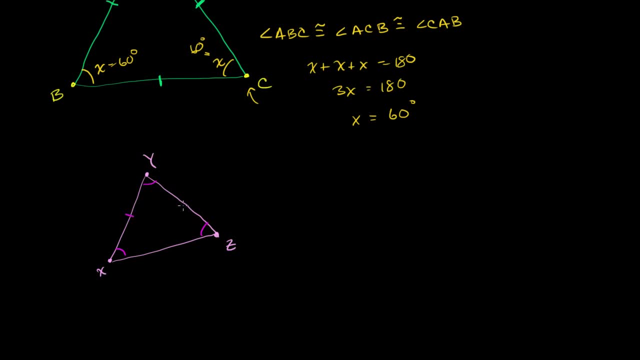 So we know, for example, that yx is congruent to yz. We know yx is congruent to yz, And we know that because the base angles are congruent. Now we also know that yz is congruent to xz. 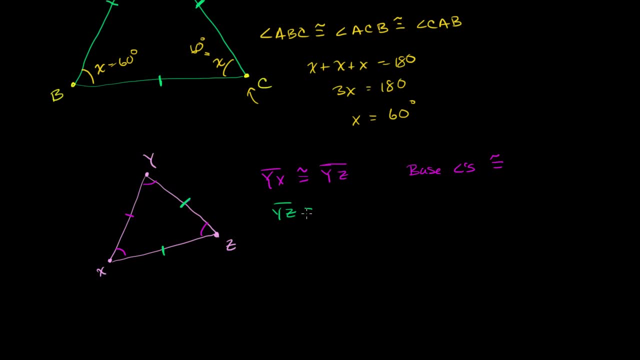 So we also know that yz is congruent to xz by the same argument, But here we're dealing with different angles. So we know that yz is congruent to xz, But here we're dealing with different base angles. So now, once again, you can view this.